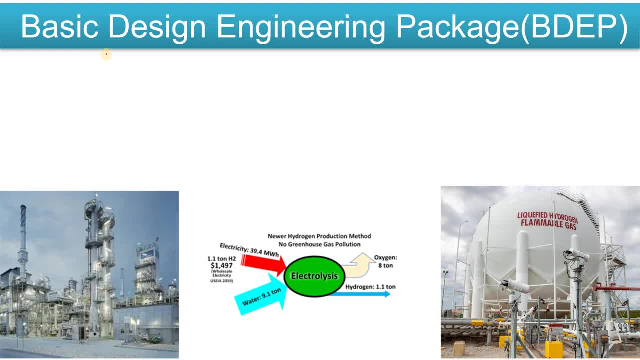 hello core engineering family. in this video we are going to discuss about the basic design engineering package that is also known as the bdep. okay, so if you want to become a process engineer or you are a new process engineer, so this video is must for you, right? because if you 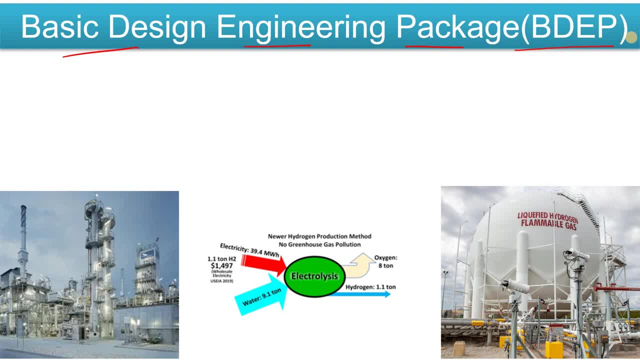 join any process engineering company or any engineering, procurement and commissioning that is epc company, then you will find out that we prepare a one package. there is a set of documents which we prepared, right? so what documents we prepared that time? what is the significance of that documents that we are going to discuss in this video? that video is very, very important if 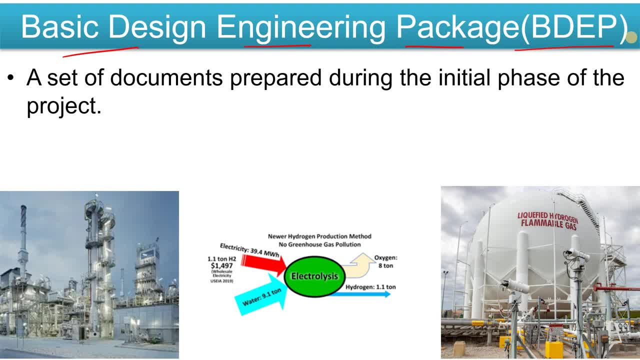 you want to become a process engineer or chemical process engineer, so please watch that video completely so that you could get to know about lots of documents and their significance, right? so first of all, let's discuss about that. what is the bdep? so bdep is basically a set of document. 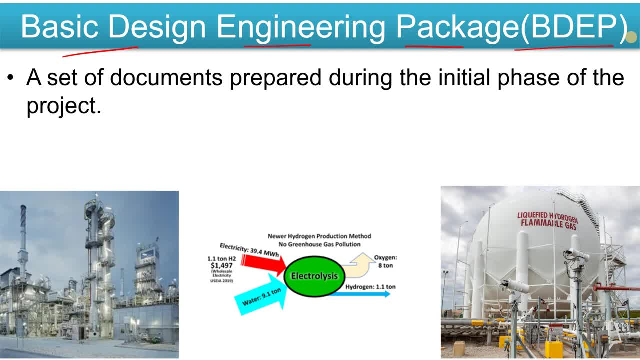 that is prepared during the initial phase of project. okay, let's suppose your company wins a project. okay, that is 60 mtpd hydrogen manufacturing plant. okay, for that plant, let's suppose you have to do the engineering, procurement and commissioning. are you getting my point, what i want to say? okay, so please let me in the comments box: what is the bdep? 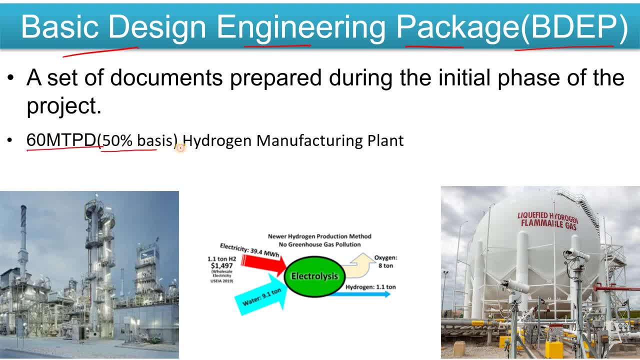 the meaning of the 60 mtpd 50 basis. what will be the capacity when i'll write that 60 mtpd 100 basis? this is the homework for you, all right? so a process engineer will prepare a bunch of documents during the initial phase of the project. that documents, or that bunch of documents. 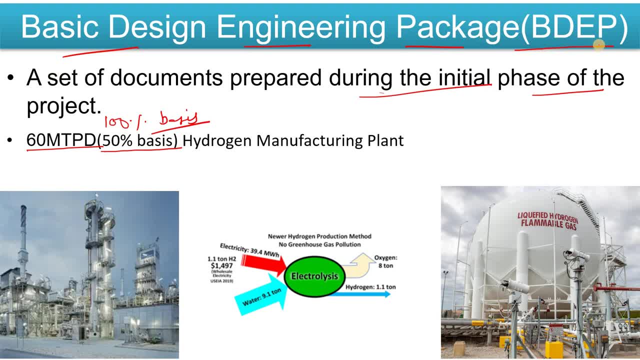 is called the bdep, that is, basic design engineering package. are you getting my point? what i am? what am i saying? okay, let's suppose there was the kickoff meeting and you collect the documents. that is the side condition which you could simply ask from the client: local norms which is used in their plant or their locality. power availability. 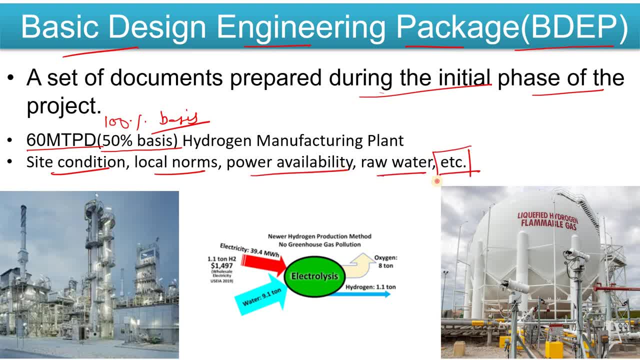 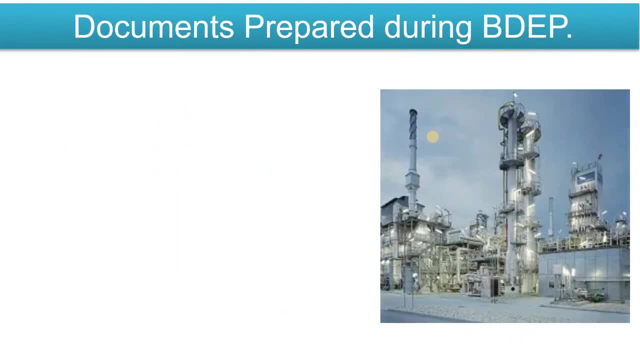 raw materials, etc. whatever the your like requirement. you could ask or you could simply get the details from the client. now, what you will do, if, what a process engineer will do. he will prepare the basic engineering design package documents. okay, so what are the documents that we are going to discuss in this video? so the first document which you will prepare, that is the. 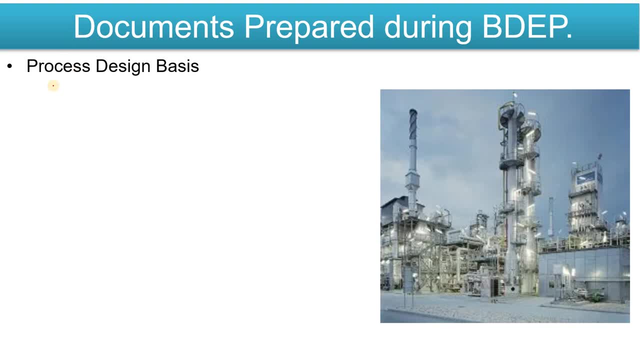 process design basis. okay, in this process design basis you will define the project, you will define the process description. in that document there is the lot of the information about the site: condition, raw material specification, product specification. then there will be the design and codes. there will be the scope of supply there. 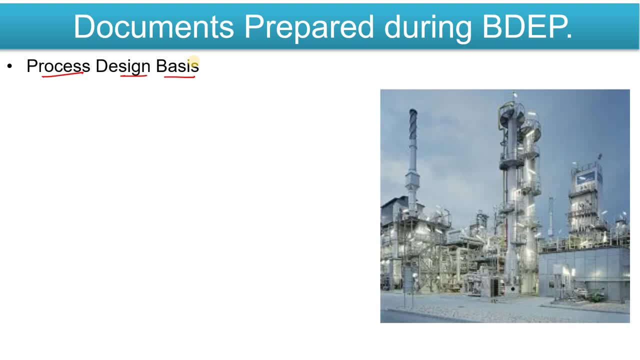 will be the side condition and most of the, the complete overview about the your process, about the electrical, about the piping, about the electrical, about the instrumentation, complete overview will be in the this process design basis. i hope you got the point what i want to say. then you will. 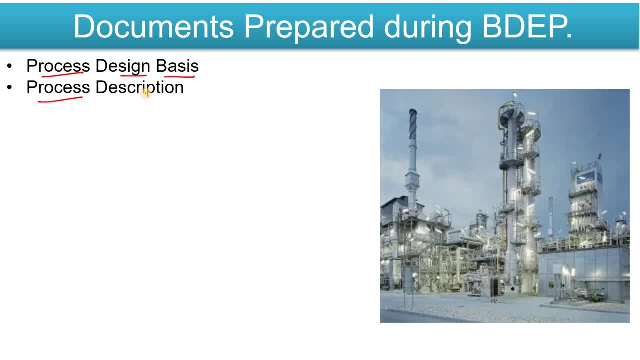 prepare the one detailed document that you will use in this process design basis and then you will prepare the one detailed document about the process description. in the process description you will only discuss about the process. description means how your process will work. what is the technical how of the process? what is the work of the each equipment that you are going to discuss in this? 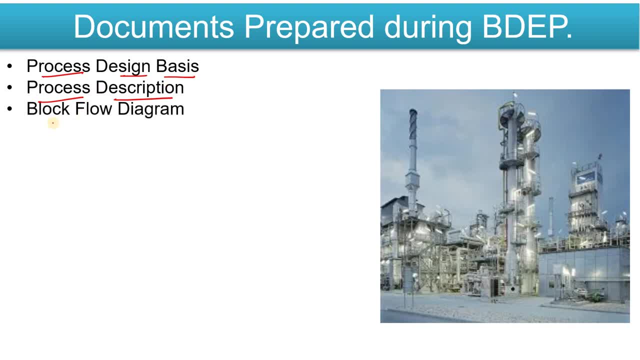 video. right, then you will prepare the block flow diagram. okay, what is the block flow diagram about this? i have already uploaded the one video. you could simply check it out, if you want to check it out in the process engineering playlist. okay, so in the block flow diagram, what you will do, you will. 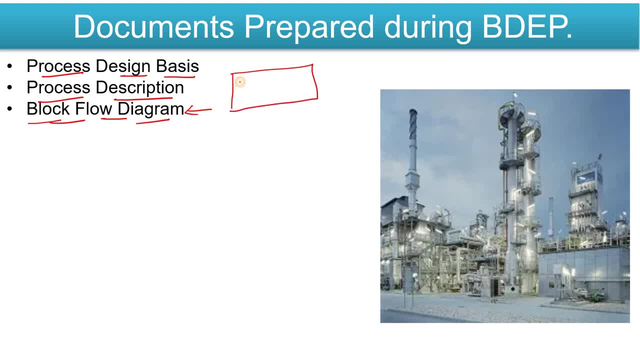 summarize the complete plant into the blocks. okay means if, let's suppose if there is any newcomers, or let's suppose if there is anyone who is not from the technical background so he could also understand that what you are manufacturing and how you are manufacturing, okay, so this is the 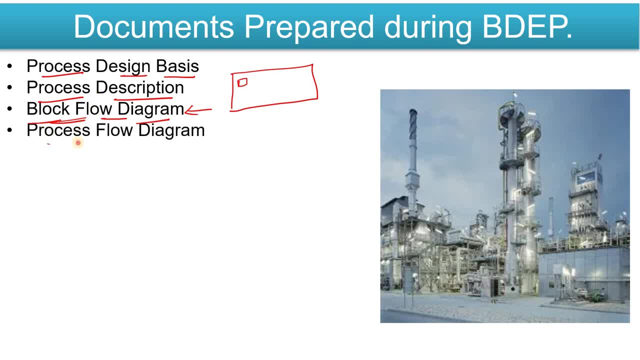 block flow diagram. then you will prepare the process engineering playlist, so in the process process flow diagram. okay, so this is the one step ahead from the block flow diagram, in that what you will do, you will simply show the equipment as well- okay, equipment as well as the critical control walls you could show here and simply 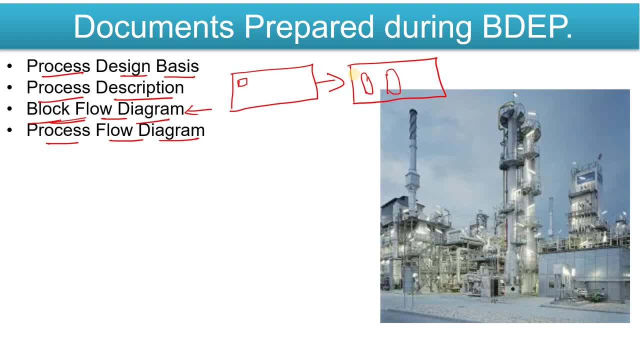 the incoming and outgoing lines or the process line you will show here right, and after that you will prepare the heat and material balance. okay, let's suppose if this equipment is here and you are, image is clean. from this equipment, the something is coming and something is going to out, then the basis and the how much amount of what Entonces impone y algo que viene. 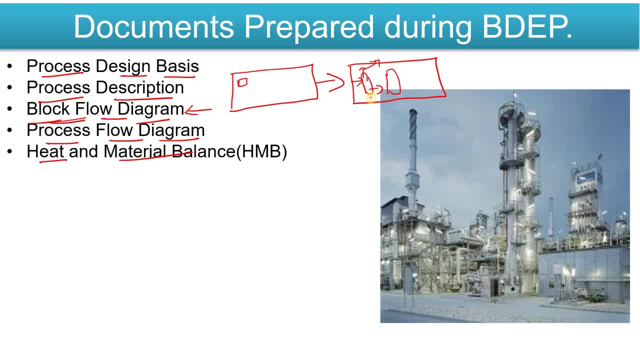 of lo que nos viene de aquí? cuánto de adalah el líquido or low-grade que reciben de la base? okay, actually, this heat and material balance is very, very important for you. actually, este heartbeat which gives us the information about the quantity, which nos da la información por la cantidad, how much quantity you are going to smallerace a cantidad que vas aballs телефonic entre las tantas y cuántas dos. 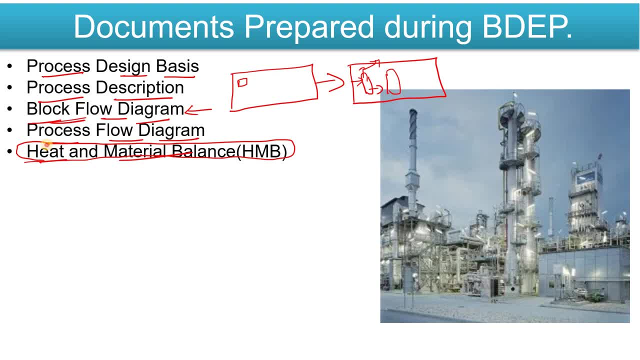 about the quantity, how much quantity you are going to feed and how much quantity you are. you are, you are getting from the top or from the bottom. are you getting my point? what i want to say then? so in the color coding document? actually, this document gives us the information about the 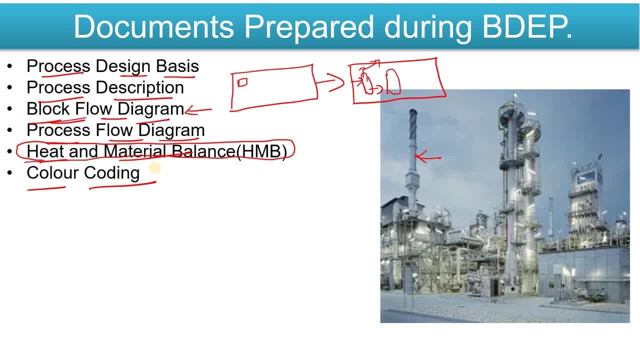 about the color. okay, like which color you have to do in the equipment, okay, what is the rl code of that color? okay, and which color you have to done in the structure, which color you have to done in the support in the piping. that's all information is you could get from the color coding, okay. 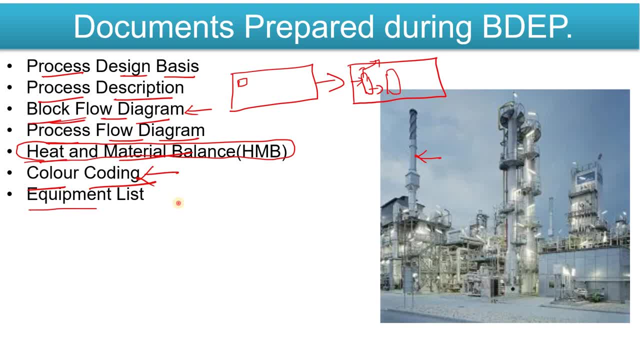 then the equipment list: okay, in your complete plant, which equipments you are going to use, what is their capacity, what is the size, that all information you are going to list in this equipment list. there, mainly there will be the vessels, okay, okay. pumps, okay, like, uh, the instrument parts will not come in this equipment list. okay, the vessel pumps. 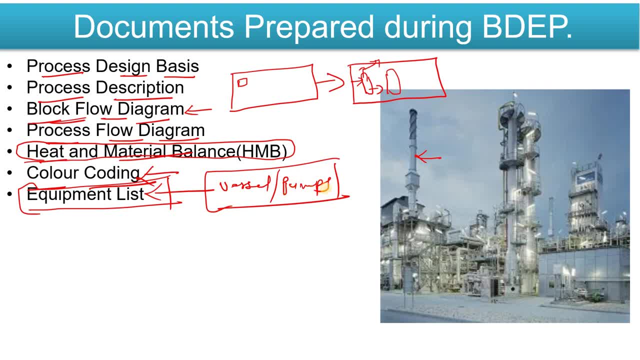 mainly will become within this equipment list, right then. next is pnid. okay, that is the piping and instrumentation diagram and which is also known as the heart of the process. so initially, you prepared the block flow diagram. okay, and for and after the block flow diagram, you prepared the 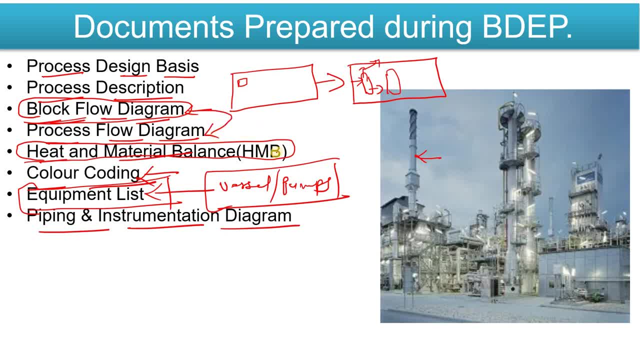 process flow diagram, that is pfd. okay, and after the simulation and and after the heat and material balance and simulation, we prepared the piping and instrumentation diagram that is also known as the pnid. okay, so this pnid is the heart of the process. okay, the one of the most important document that 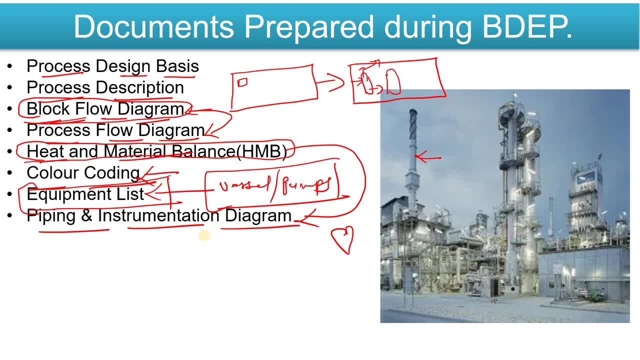 is pnid? why pnid is very, very important? because from the pnid only you could get to know that which equipment is where means: all the detailed information will be there, like about the instrument, about the equipment, about the pipeline. everything will be there, excluding something that we will discuss later. 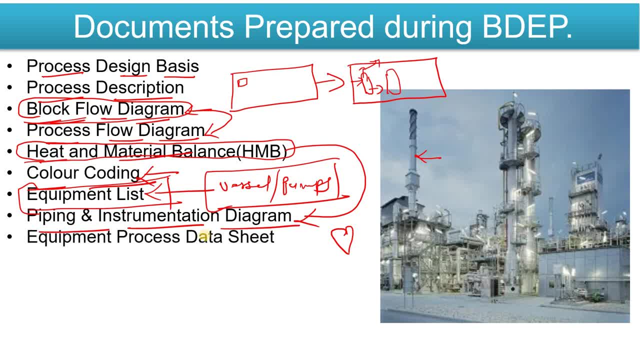 right after that we will prepare the equipment. process data sheet means you will prepare about the each equipment. whatever the equipment you are going to use, you will prepare the process data sheet of that equipment. like, let's suppose, if this is your one, one vessel, then you will prepare. 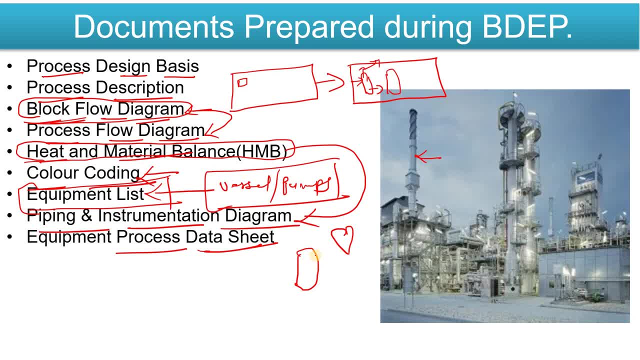 the process data sheet of that vessel, about the. you will give the information about the nozzles, about the nozzles, about the dimensions, about the codes. you also provide the design temperature, design pressure, operating temperature, design temperature, right. so these information is provided by you and that process data sheet will be prepared by the process engineer. 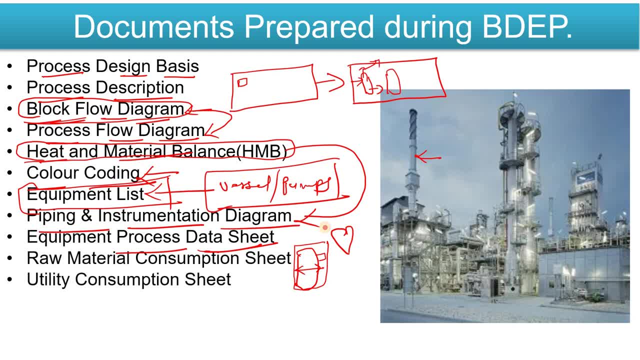 okay, Then we also gave the raw material consumption sheet, utility consumption sheet. Then we prepared the. after the completion of the P&ID, you could prepare the instrument process data sheet means about you will prepare the process data sheet of the control wall level transmitter pressure transmitter- PRV, TSV, PSV, AFR. 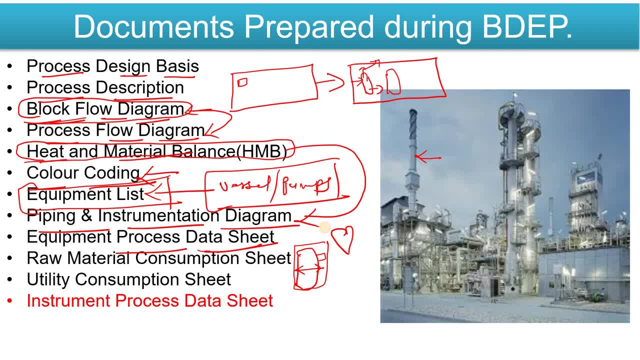 So all the instruments detail you have to prepare within the instrument process data sheet. Then you will prepare the piping process specification. So in the piping process specification means there will be the lots of pipes will have a different application, There will be a different MOC. 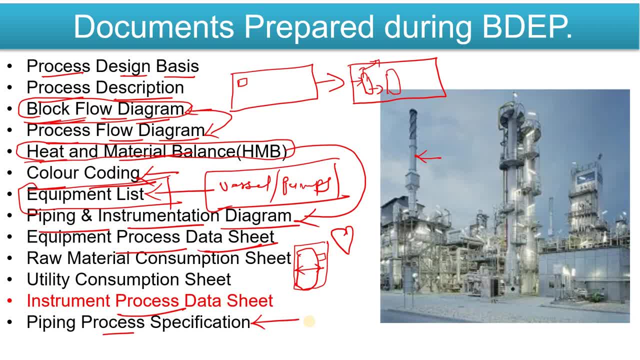 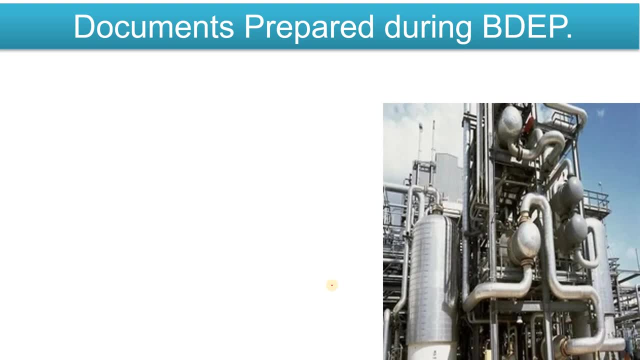 There will be the different operating temperature: design temperature. operating pressure, design pressure. OK, so that information is provided in the piping process specification. Then same we do for the wall process specification, because each wall will have the different MOC, Different application. there will be some wall which would be used in the cooling water line. 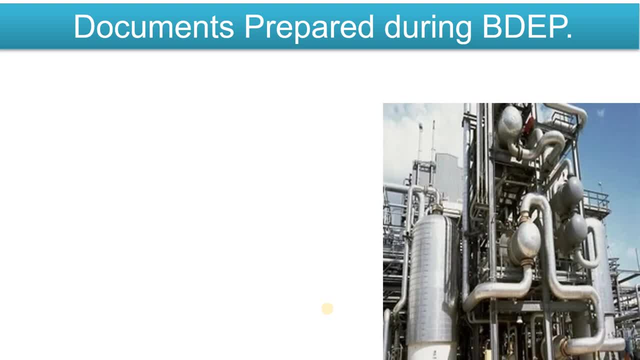 There will be the another wall that will be used in the hydrogen line. OK, there will be the other walls that will be used in the airline, So on. So there is specification there. operating temperature code: operating pressure: design temperature: design pressure is given in the wall process specification. 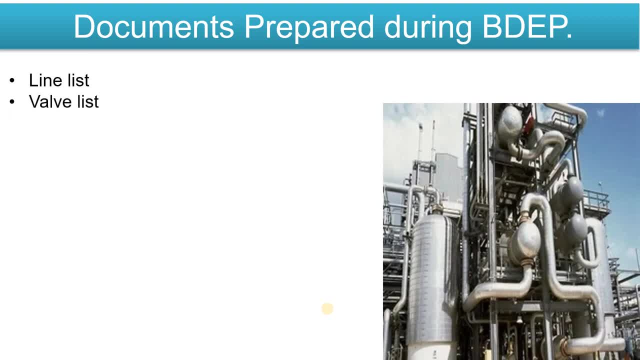 Then we prepare the line list, then we prepare the wall list. So in the line list we provide the information about the each line. OK, so like, like how, from where this line is coming and where that line is going. So each line has a different name, different code. 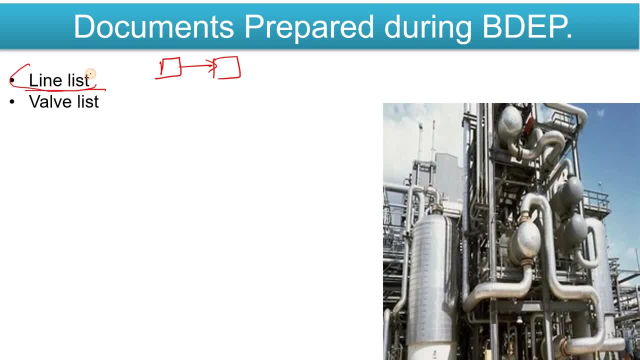 And in that line list you could get to know about the, about the MOCs. OK, then, with the help of the P&ID, the wall list will be prepared and from the wall list, wall summary will be prepared. OK, how much? 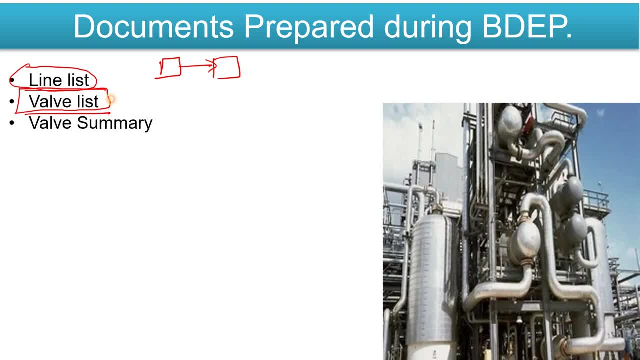 What type of wall you are like you have to purchase, which type of the walls you have to purchase, what will be the end connection of the data was complete detail you will get from the wall summary. Then there is the another document, that is, the insulation specification. 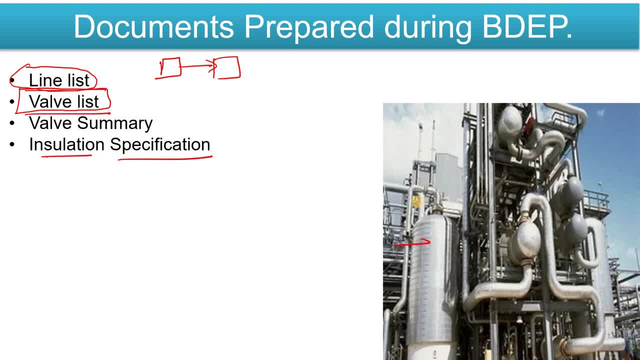 If the insulation is using in your plant or in the equipment in the line, which type of the insulation you are going to use. that is like whether it is cold insulation, whether it is hot insulation. What is the thickness? Everything You have to cover in this specification: see specification document. then the process control philosophy. 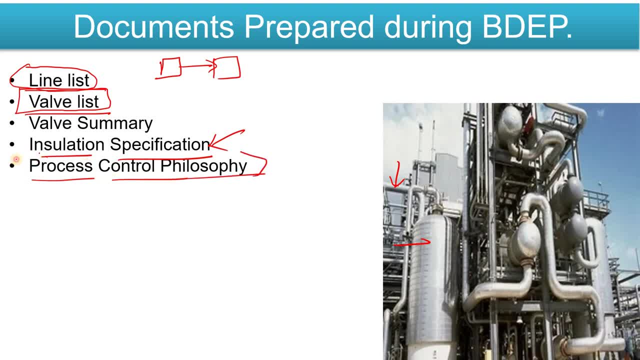 OK, that is also prepared by the, your P&ID. These all documents are prepared with the help of the P&ID, So that's why I say that the P&ID is the heart of the process, Right? What information you provide in the process? control philosophy? 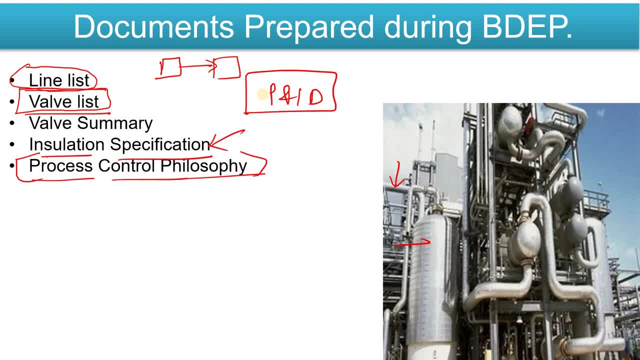 So actually in the process control philosophy, whatever the interlocks which you have given, whatever the LTEs you have given, whatever the alarms you have given, So everything is included in the process control philosophy means how your process has to be controlled. That information is provided in the process control philosophy. 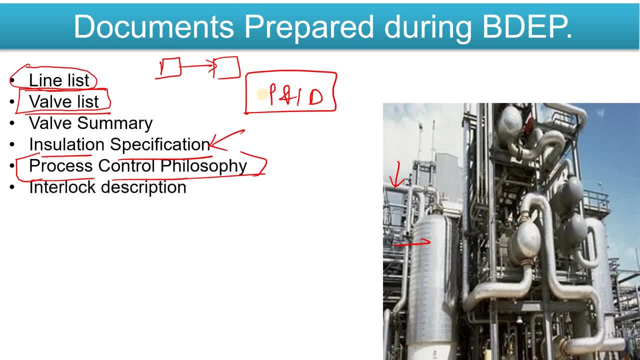 Then interlock description. OK, let's suppose if you have your pump has to be tweaked with the PT, that is, from the high, high pressure. or let's suppose it could be with the low, low level of the tank. OK, so that all information is provided in the interlock. 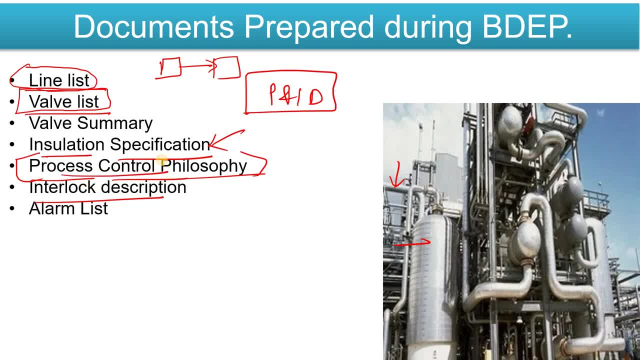 OK, so that all information is provided in the process control philosophy. Then there is the alarm list. Let's suppose, if there is the one, LTE, and that LTE has the three and four alarms. Let's suppose that high, high, high, low, low, low. 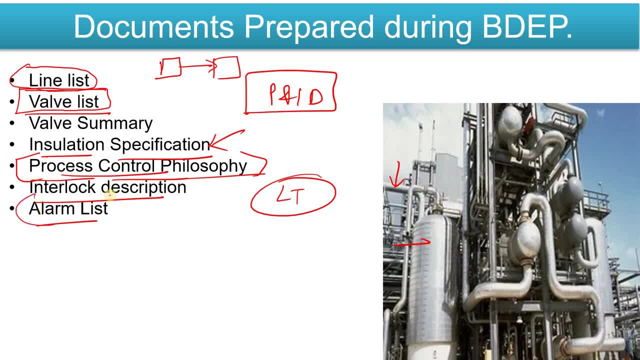 So at which point what alarm will come? That information is provided in the alarm list. Then hazardous area classification. OK, so that document is also very important if there is the hazardous area classification. So what Area will come in the zone one, zone two, zone three? 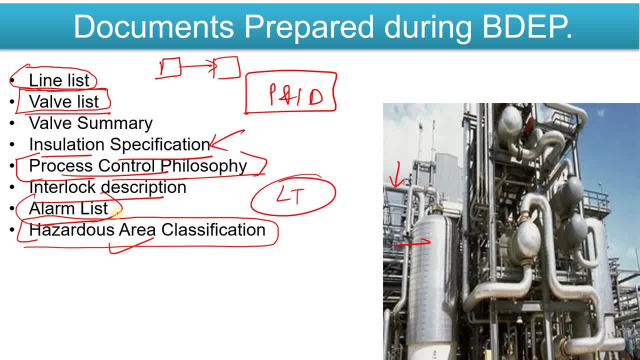 So that all information is provided there. And also that document is also very, very important with respect to safety as well. Right, Then we prepare the DCS graphics that also for that document Also P&ID will be referred, Then operating manual, how your plant will be run. 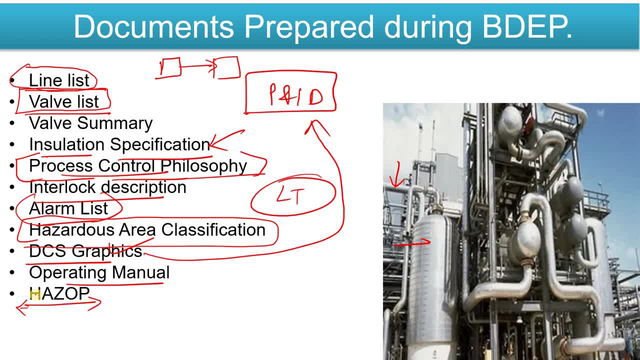 HAZOP, if in your process or if you have to do the HAZOP. So that is also very, very important. In the HAZOP, what mainly we do we check, that is, our P&ID is OK or not. 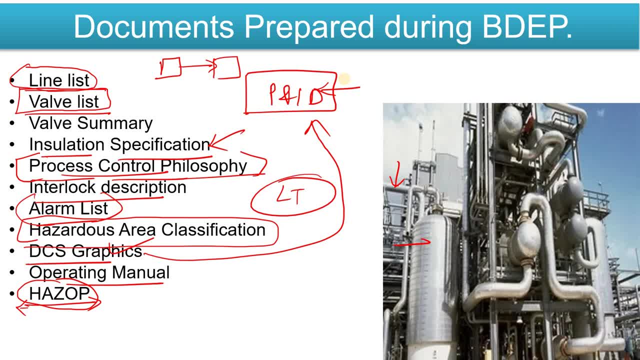 Is our plant which we are proposing. that is OK or not. with respect to safety, OK, if there is anything comes, then we include that in the P&ID or in our design consideration Right. Then the site condition document. that is the initial document, which is also very, very important. 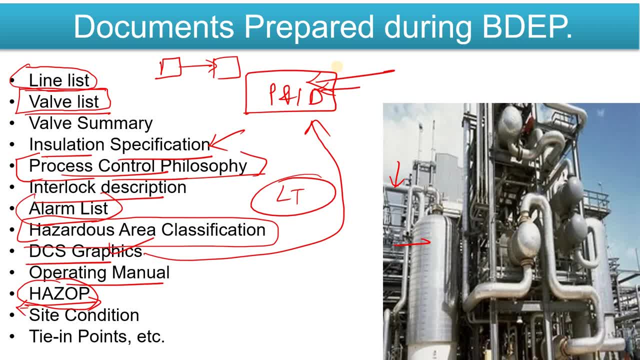 And in the last, that is, the time points. OK, There could be the other documents as well, like your whole point list, etc. But these are the major documents which is prepared during the basic design engineering package And after that the detail engineering comes into the picture.